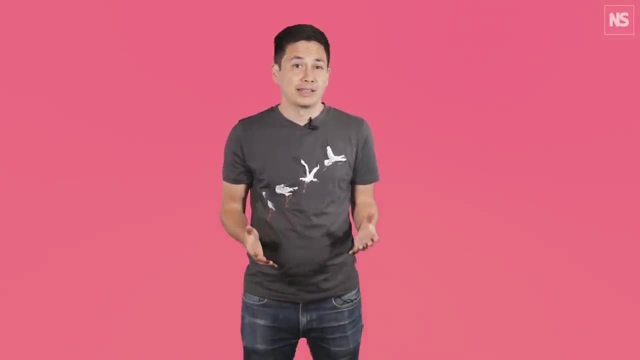 it's a bit of a molecular jack-of-all-trades. So it seems to be a good idea to use DNA as a way of storing information and it's not a good idea to use DNA as a way of storing information. So it seems more likely that the first life forms were based on RNA and that DNA and proteins came later. The trouble is in the lab. we find that RNA needs a lot of help to assemble or copy itself, So chances are it wasn't enough to start life on its own. As far as we know, life can't exist as chemicals in a soup. 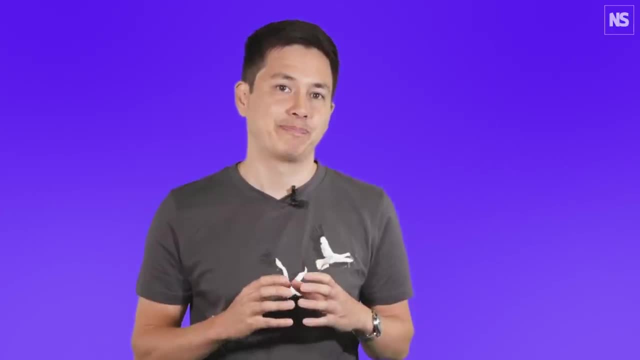 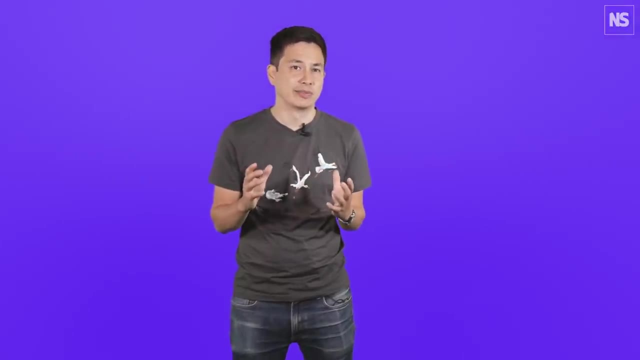 All the living things we know about are made of cells that package up the chemicals. Some scientists reckon that the first organisms were made of oil droplets or bubbles that acted like primitive cells, providing the structure for life to get going. In the lab, we can create droplets that show life-like behaviour, sensing and responding. 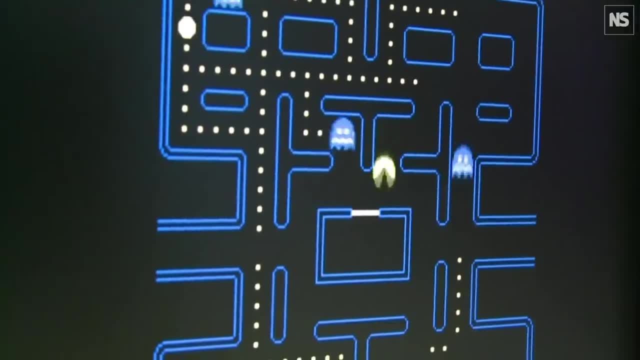 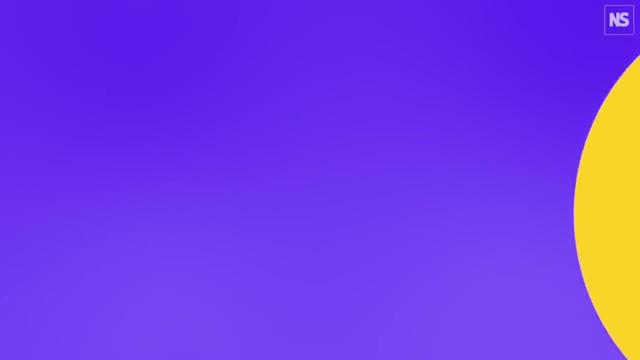 to their neighbours and moving towards food sources, A bit like Pac-Man. Crucially, though, these droplets can't replicate or evolve, meaning it's unlikely that this guy was your ancient ancestor. Finally, it's been suggested that life began with chemical reactions that extracted energy. from the environment and used that energy to build the molecules of life. In other words, metabolism came first. This might have happened in hydrothermal vents at the bottom of the ocean, where energy from inside Earth heats the water up to 400 degrees. 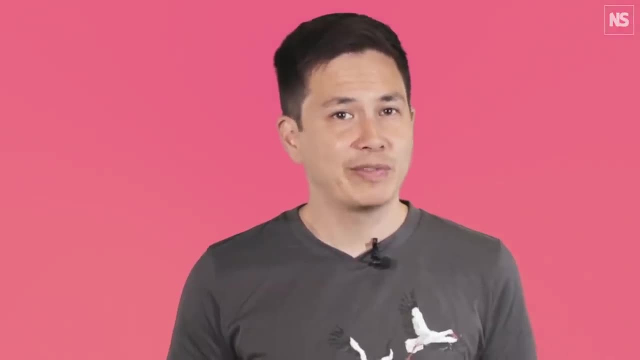 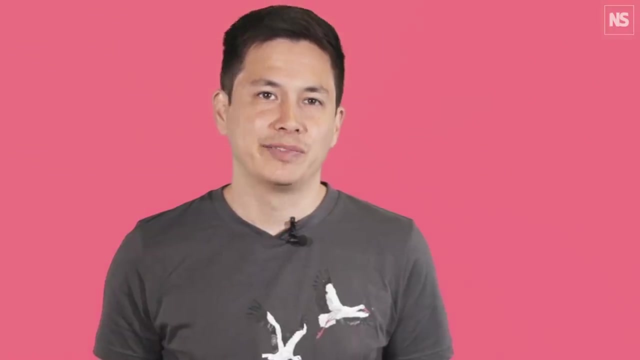 So which came first, cells metabolism or genetics? It's a bit of a chicken-and-egg conundrum. When any of these theories are tested out in the lab, none of them produce anything remotely life-like. The alternative is that life arose fully formed with all of these elements in place, right? 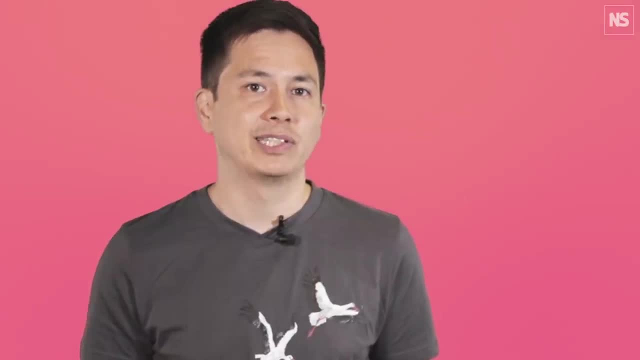 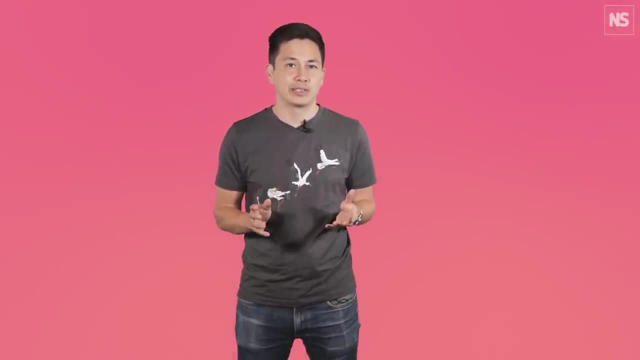 at the start That might seem even more unlikely, but recent evidence has led some scientists to think that's exactly what happened. The chemistry required involves ultraviolet light and periodic drying, so the most likely location for this is thought to be chemical-rich soil. 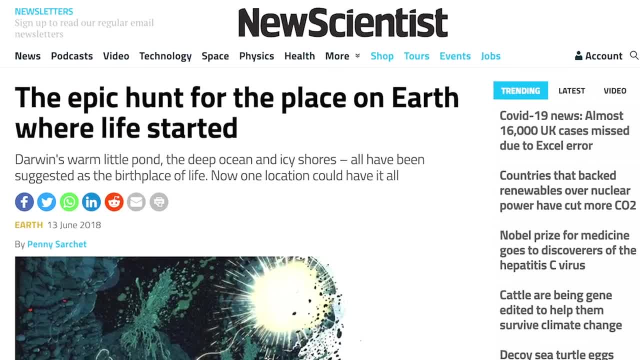 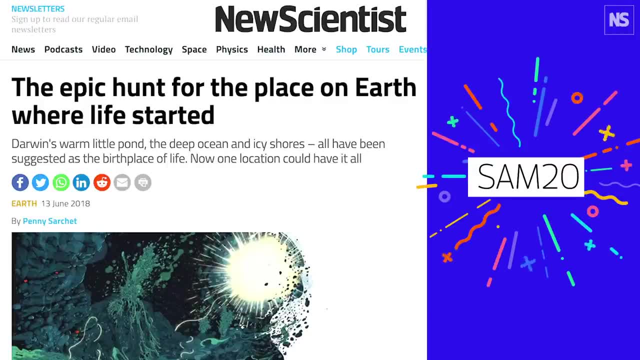 So what's the answer? You can read more about that idea in New Scientist. If you'd like to subscribe, we'll give you 20% off if you use the code SAM20.. So the origin of life is still shrouded in mystery. 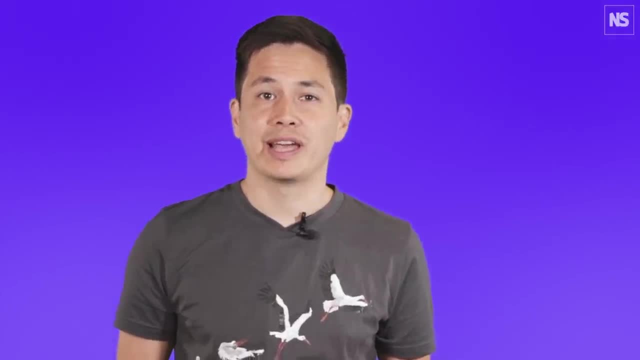 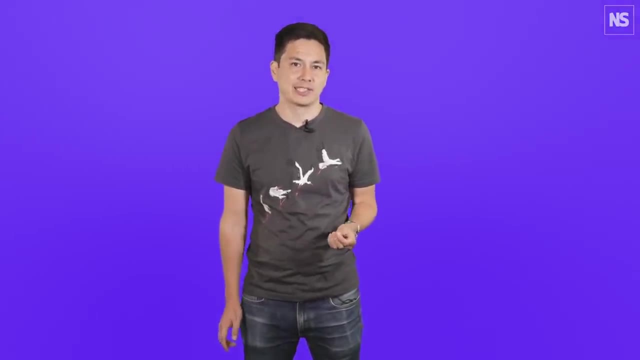 Scientists have tried all sorts of experiments to recreate life. They haven't gone all the way yet, but we've made a lot of progress. Maybe one day soon we'll succeed in creating artificial life in the lab, which could tell us how our oldest ancestor came to be. 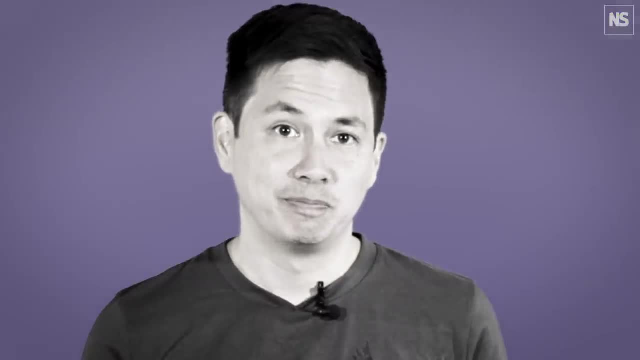 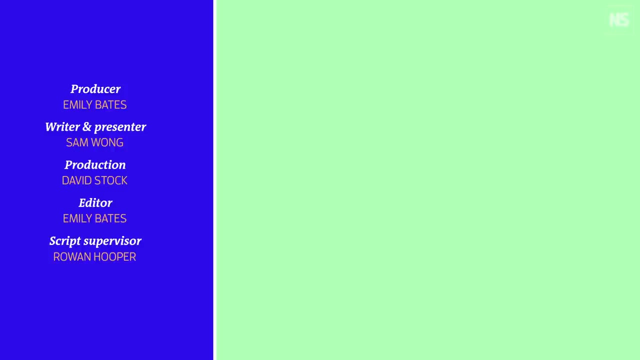 What could possibly go wrong. We'll find out in the next episode of New Scientist. Thanks for watching. We'll see you next time. Bye.